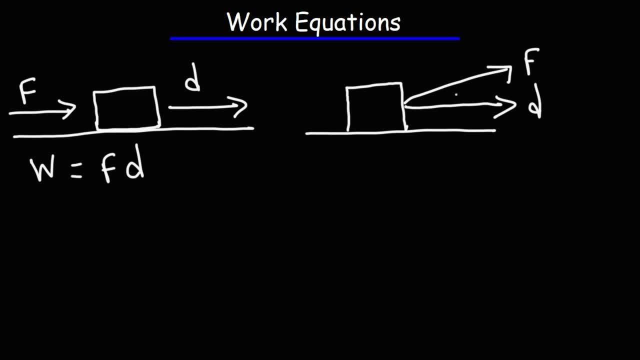 so the displacement vector is along the x-axis And theta is the angle between the force and the displacement vectors. We can calculate the work done by this force using a variant of the dot product formula which is fd cosine theta. So if you know the angle between the two vectors, all you need is the magnitude of the two vectors times cosine of the angle between them. 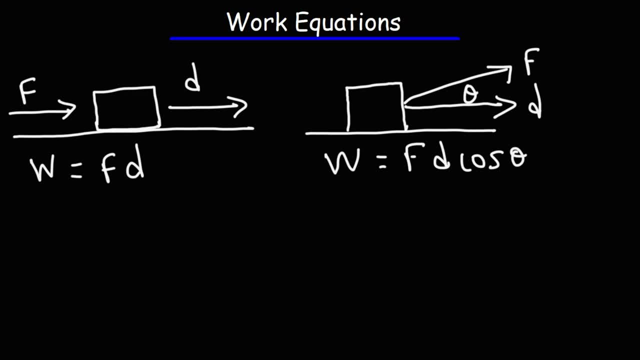 and that'll give you the work done by theta. Now let's say, if you have the force vector and the displacement vector, but you don't know the angle between them, but you know the components of those two vectors, Well, you can calculate the work done by that force by using the dot product formula. 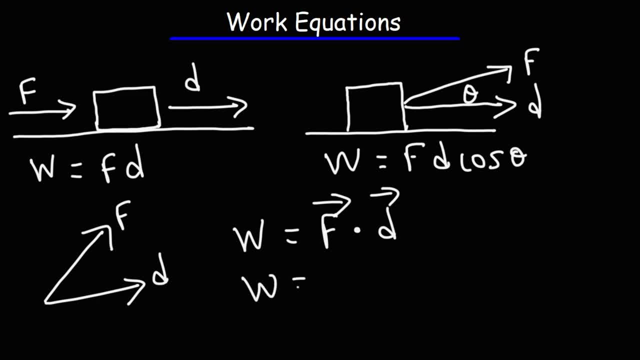 So it's the dot product of those two vectors, which is you're essentially multiplying the x components together along with the y components together. This will give you the work done in the x direction, and that'll give you the work done in the y direction. 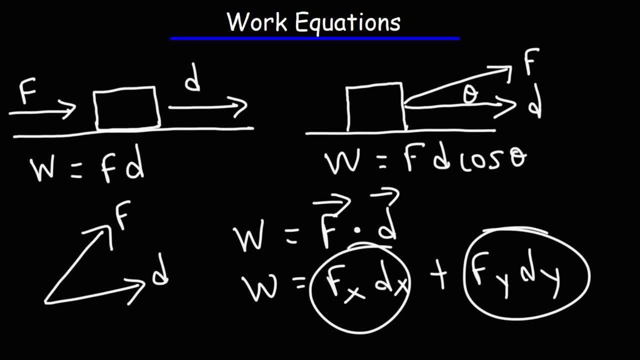 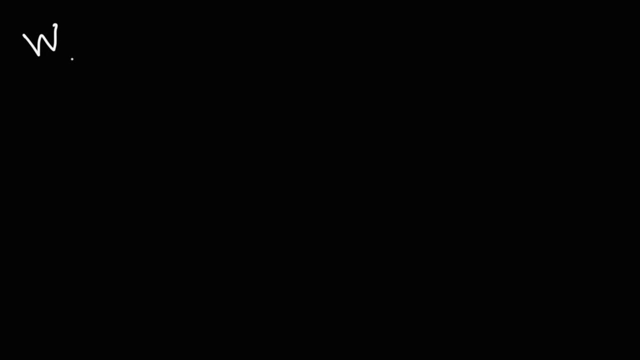 Since work is scalar, you can just add them together to get the total work done by that force. So that's how you can calculate the work done by a force. Now, work is also equal to the change in kinetic energy. The work done by the net force acting on an object is equal. 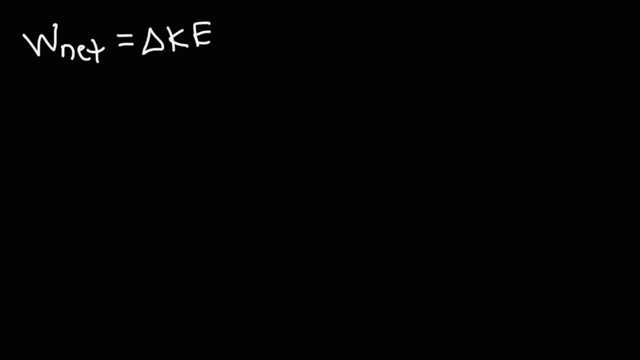 to the change in the kinetic energy of that object. This is known as the work energy theorem. Now, kinetic energy is one half mv squared, So the network is going to be the difference between the final and the initial kinetic energy, which will simplify to this formula. 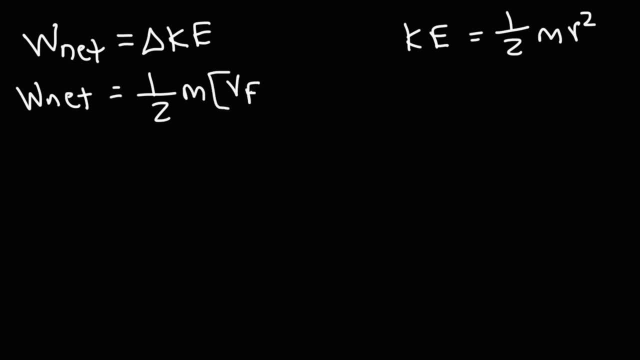 It's going to be one half times the mass times, the square of v, final minus the square, And that will give you the work done by the net force on an object, Now the work done by conservative forces like gravity, the electric force or the restoring force of a spring. 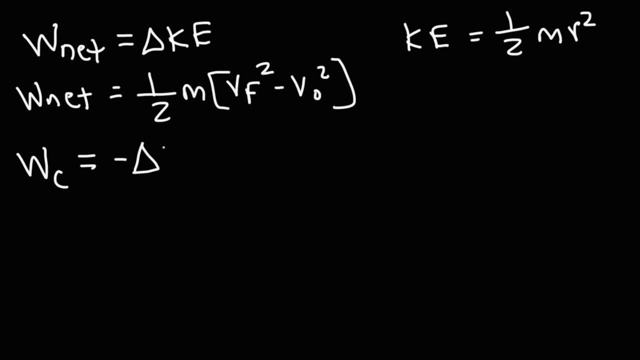 this is equal to negative of the change of the potential energy of the object. Gravitational potential energy is equal to negative of the change of the potential energy of the object. You can also see it this way, mgh as well. You can get the same result using both formulas. 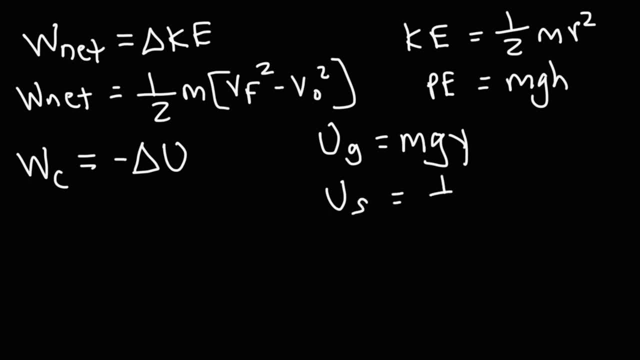 The elastic potential energy stored in the spring is one half kx squared. So let's say, if you want to find the work done by gravity, it's going to equal negative times, the change in potential energy, which will be mg, delta, y or y2 minus y1. the work done by the spring is going to be negative 1. 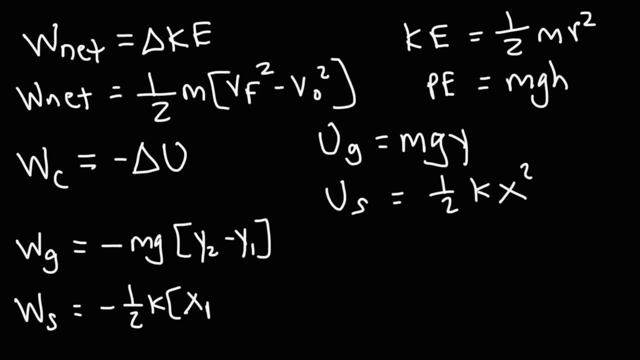 half K times X final squared minus X initial squared. so basically we're using these formulas. so the work done by a conservative force is negative of the change in the potential energy and the work done by the net force acting on an object is equal to the change in the kinetic energy of that object. 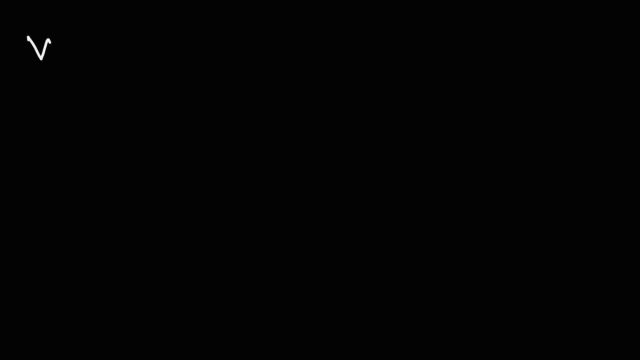 now when dealing with gases. whenever a gas expands it can apply pressure against the piston, which can move and it can do work. so the work done by a gas is negative times the pressure, times the change in volume of that gas. so that's another way in which you can calculate the work done by a gas, or just in. 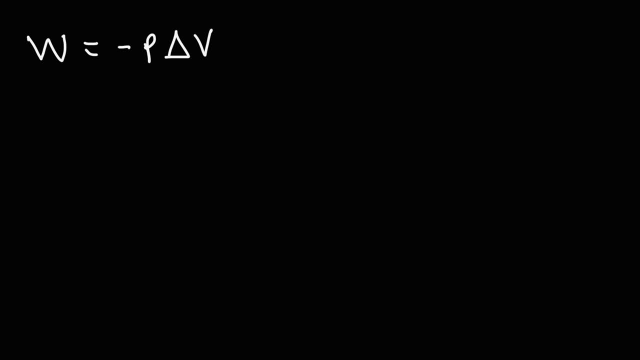 general now, power is work divided by time. it's important to understand the difference between energy and work. energy is something that an object has. an object can have kinetic energy, it can have potential energy. work is really a mechanism in which energy is transferred from one object to another. so if you think of energy as money, like 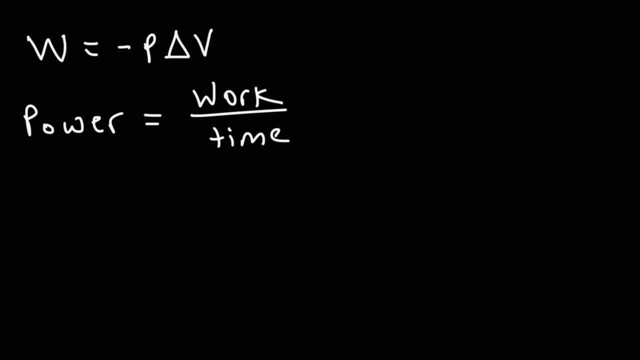 how much money you have in your bank account. work would be like the transaction, the deposits and withdrawals, the transfer of money from one account to another. so work has to do if the transfer of energy, and that energy is transferred by the action of a force acting on an object. so whenever you hear work, think of the transfer energy. whereas 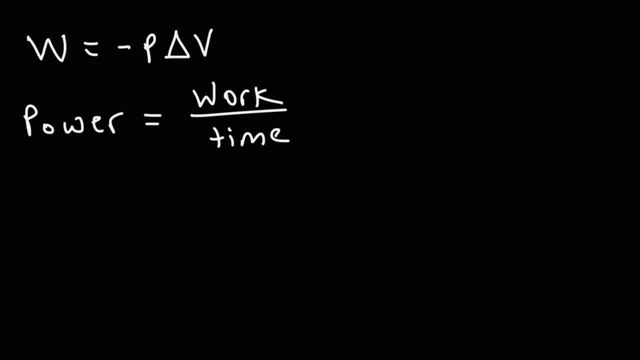 energy is something that an object possesses, and whenever an object has energy, it has the ability to do work, which means it has the ability to transfer that energy to something else. now, power is the rate at which energy is It's work. divided by time, Power tells you how fast energy is being transferred. 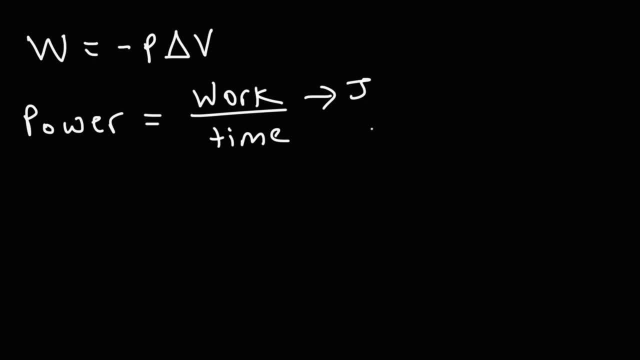 Work, kinetic energy, potential energy. they're typically measured in units of joules. The standard unit of time is the second. The standard unit for power is the watt. So one watt represents one joule of energy being transferred every second. So if you have a 500 watt generator, that means it could transfer. 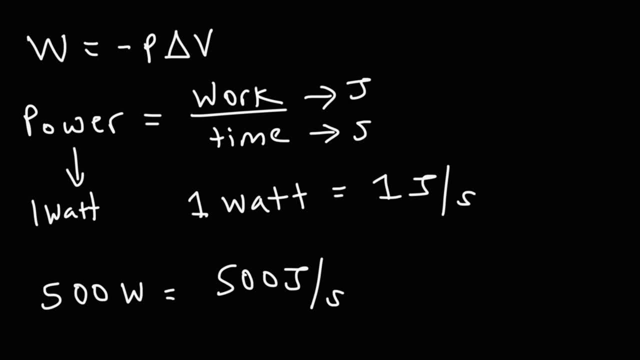 500 joules of energy per second, or it could transfer 5,000 joules of energy every 10 seconds. So that's the basic concept of power. Now you can also calculate work by multiplying power and time. You'll see other formulas that. 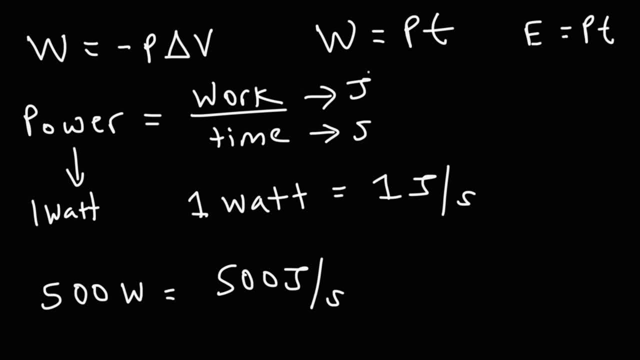 would say energy is a constant. Energy is equal to power multiplied by time. And just remember, work is just the change in energy. Now, going back to this equation, power is work over time. Work is force, times, displacement, And we know that velocity is displacement over time. 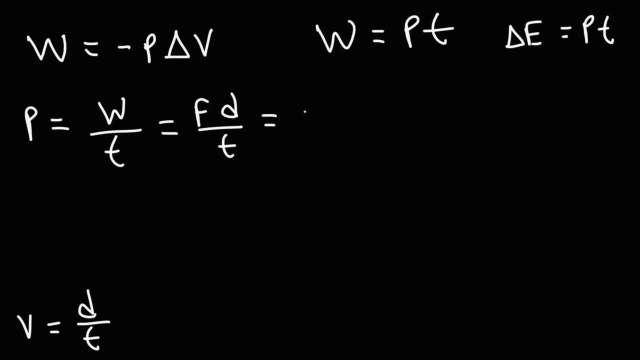 Okay, So we can replace d over t with velocity, So we get: power is force times velocity. Now we know that work is the dot product of the force and the displacement vectors, Instantaneous power, is also the dot product of the force and velocity. 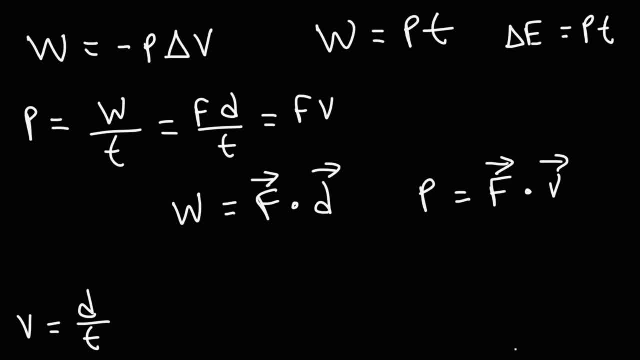 vectors. If you simply multiply these two together, this will give you average force. If you multiply force by average velocity, you get average. I said average force, but I meant to say average power. This equation here will give you the instantaneous power. 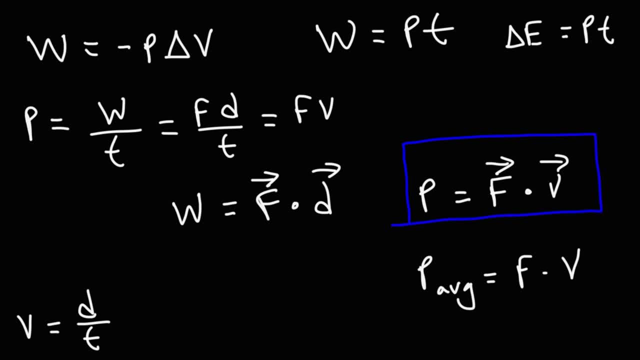 if you have the force and velocity vectors. But just remember that power is force times velocity. Now we talked about watts. It's good to know that a kilowatt hour is a kilowatt hour And if you come across this unit, the horsepower, one horsepower is 746 watts. So those are. 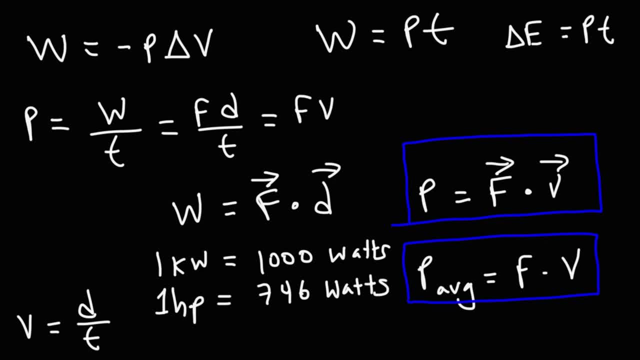 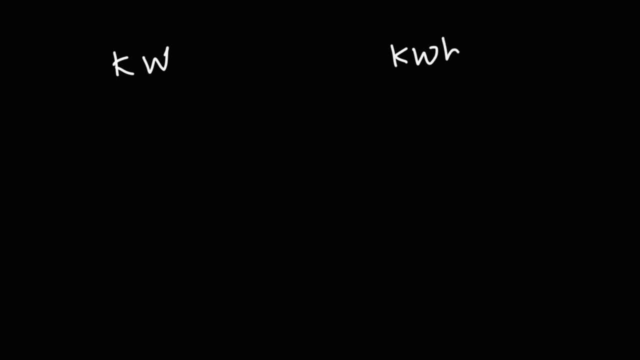 some conversion factors that you want to be familiar with Now. sometimes you'll see things like kilowatts and other times you'll see kilowatt hours. The kilowatt is a unit of power. Make sure you understand that So you can see that. you can see kilowatts, kilowatts, kilowatts, kilowatts, kilowatts. 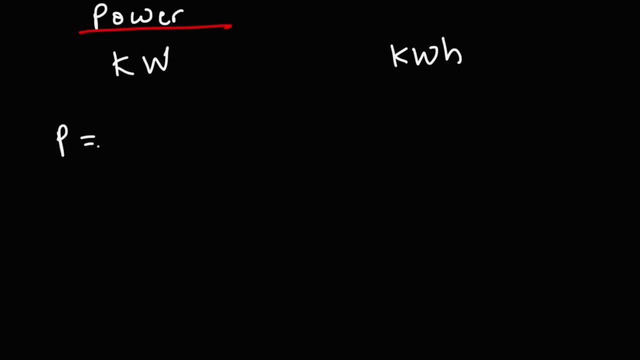 kilowatts. those are units of power. Remember, power is work over time and it's also force, times, velocity. The kilowatt is not- I mean the kilowatt hour is not the unit of power, but it is the unit. 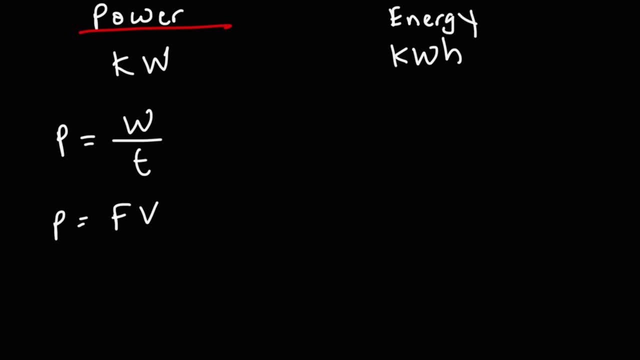 of energy. So that's what you'll typically see in your electric bill: how many kilowatt hours you've used for the month. So kilowatt has to do with power hours has to do with time- When you multiply power and time you get work- or the change in energy, which is how much energy has been transferred. 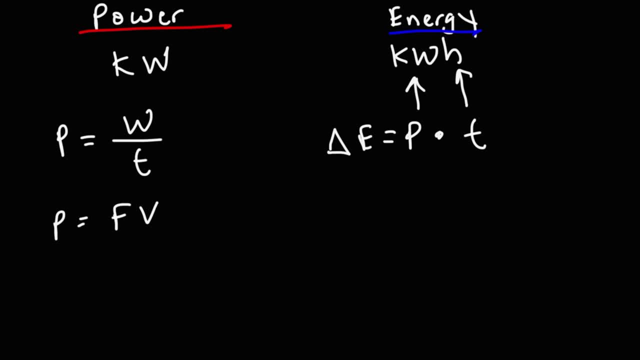 over that time period. So power multiplied by time give you the work or the change in energy in joules or kilowatt hours. So kilowatt hours, Hours, joules, these are units of energy and not power. So make sure you understand the difference between the two.